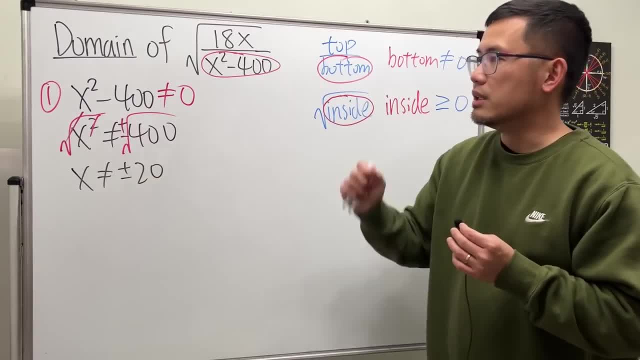 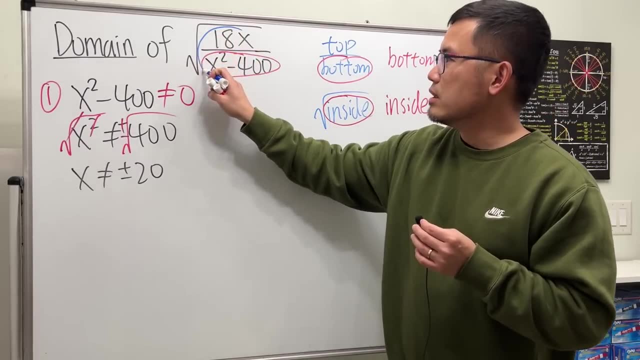 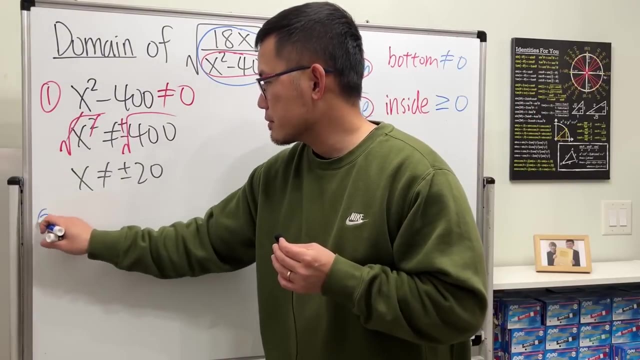 and we found two numbers that we can use for this function. Now the harder part for this question is that we have to make sure that inside of the square root being positive. So for the second part, we have to write down the inside expression. 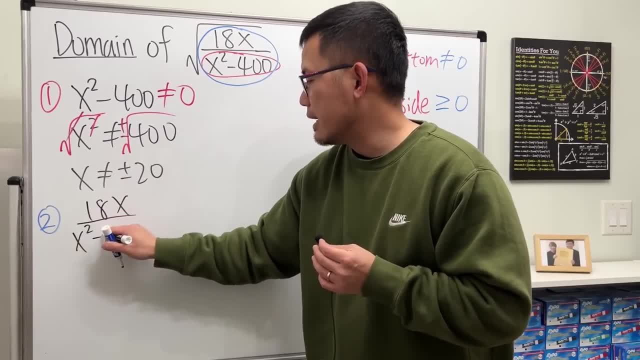 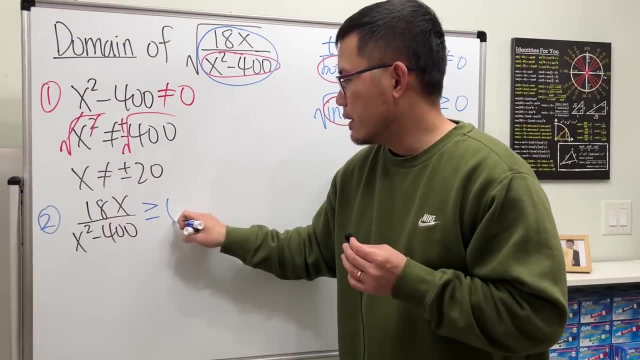 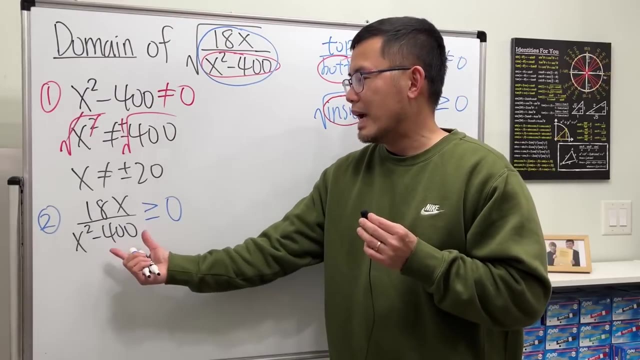 18x over x, squared minus 400.. We have to make sure that is greater than or equal to zero. So just kind of forget all that. focus on this right here And this right here. it's also not easy to solve because we have a rational inequality. 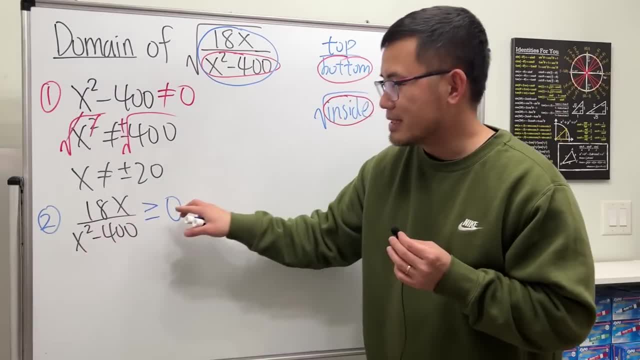 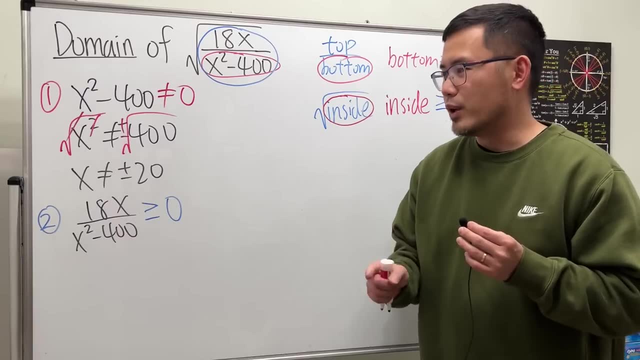 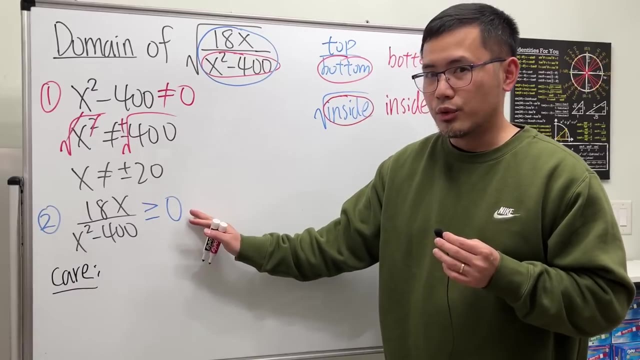 non-linear inequality. Do not just multiply this on both sides. It's not like that. So how do we do it? This is the safe way to do it. Go ahead and find out the numbers that we care. Especially the right hand side is zero already. you can proceed to do that. 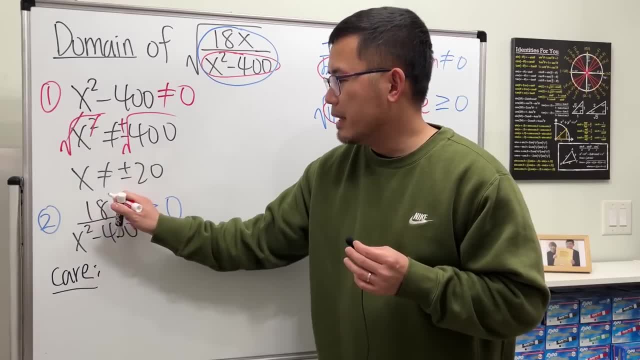 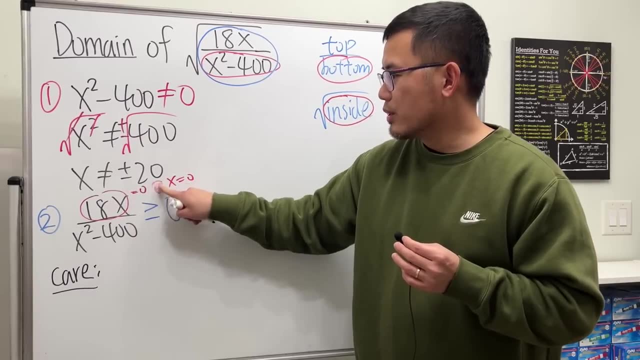 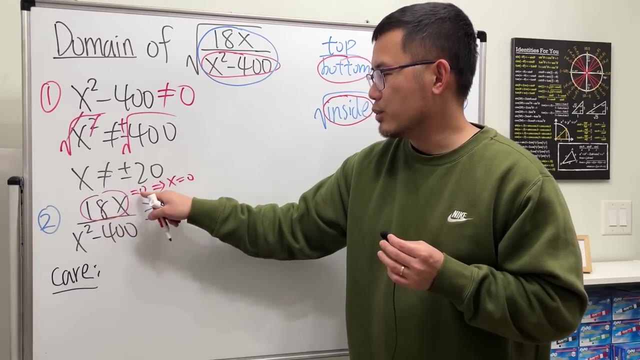 On the top we have 18x. Make this equal to zero. That implies x is equal to zero. So if x is zero, you will get a number that we care Right: 18x equal to zero. x can be zero. So we first care about zero And the next you look at the. 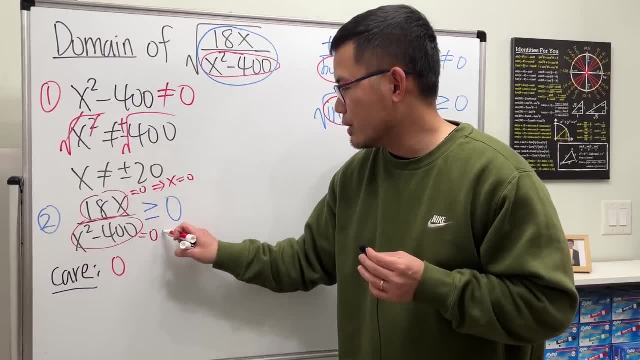 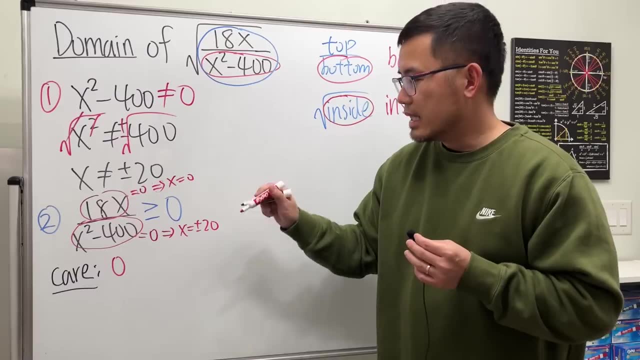 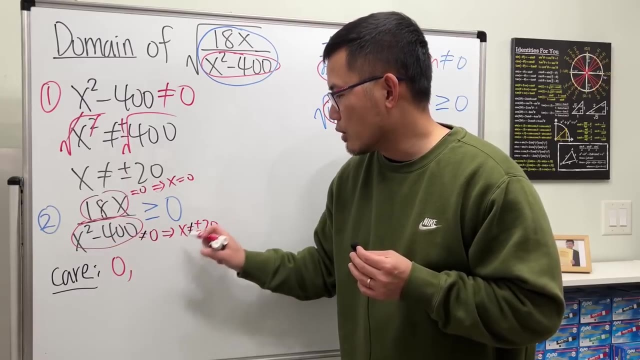 bottom, you also make it equal to zero and this implies it's the same thing. right there, x is equal to plus or minus 20.. Technically not equal because again they are on the bottom. So right here we have to care about zero and also plus or minus 20.. 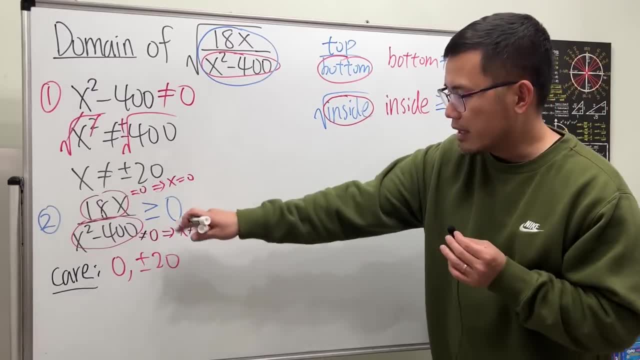 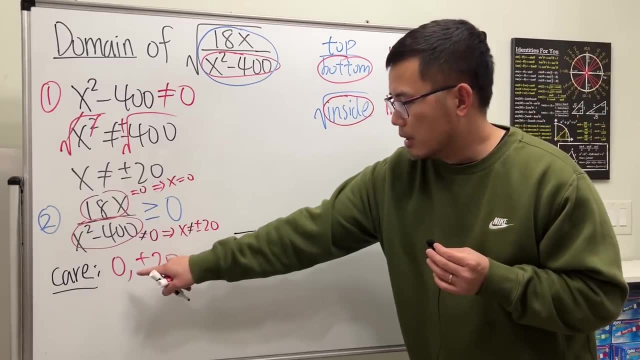 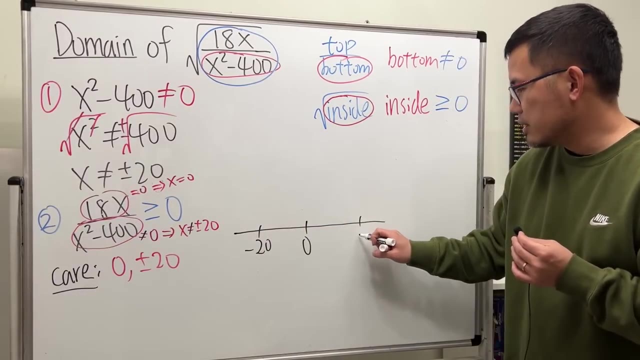 And the best way to do this is now take that and then draw a number line right here and then just test out the interval We have to put in these three numbers right here. So let's say here is zero and then here is negative 20, and here is positive 20.. 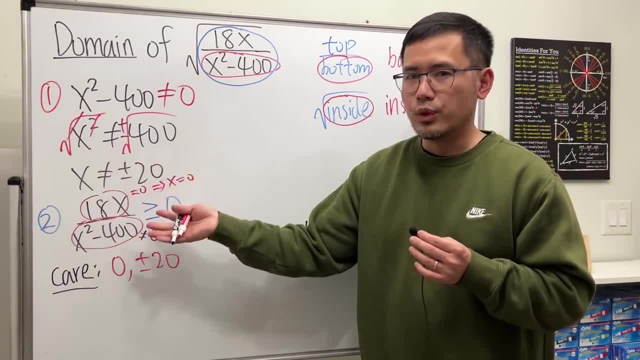 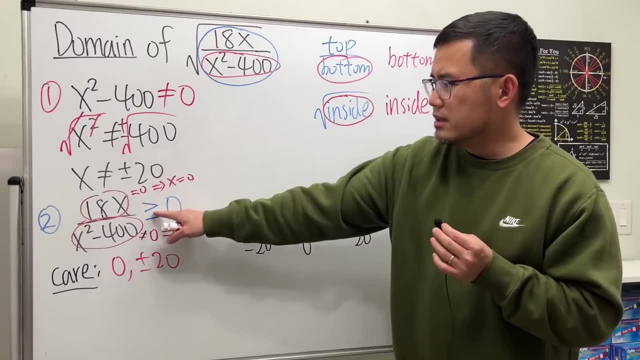 Remember we cannot have. x is positive or negative, 20. So right here I'm just going to put an open circle and open circle, and because this is a greater than or equal sign, that means x could be equal to zero, So zero is included. 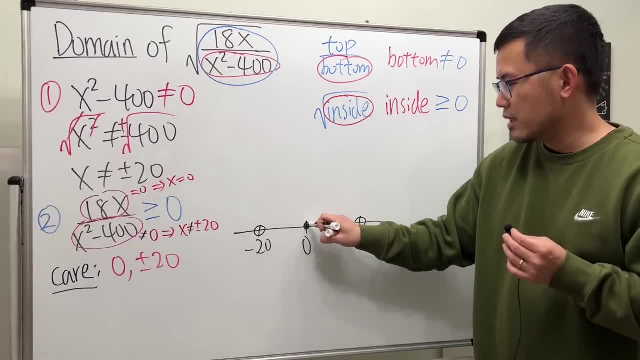 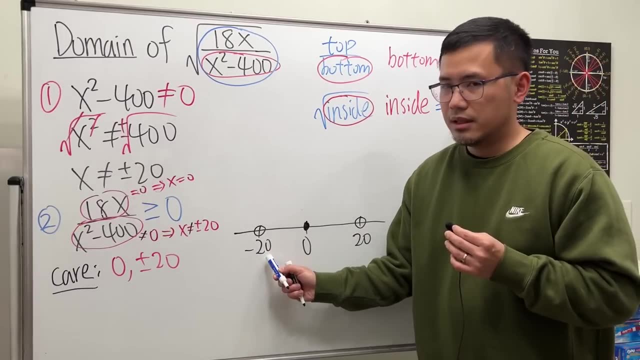 So you can circle, put close circle right here like that. Now test it out: How Pick a number less than negative 20. So let's just go ahead and say negative 21. Don't be too fancy, right? 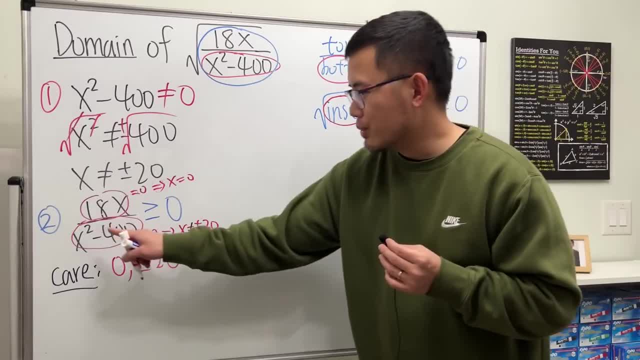 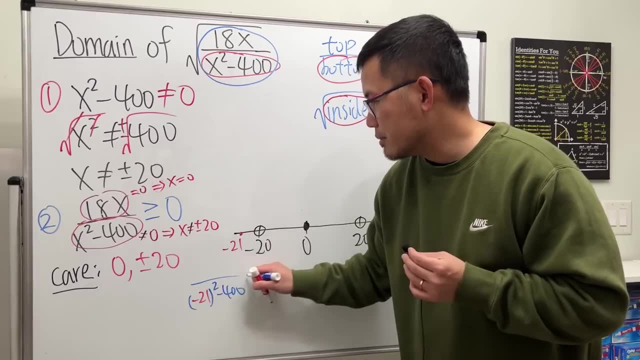 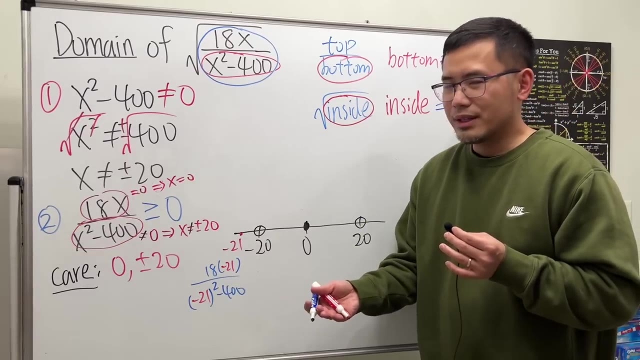 Let's say negative 21. And then just plug it into this right here. So we have negative 21, and then squared minus 400, and then the top is 18 times negative 21. And you don't really have to work out like specific numbers, You can just test out if it's positive or not. 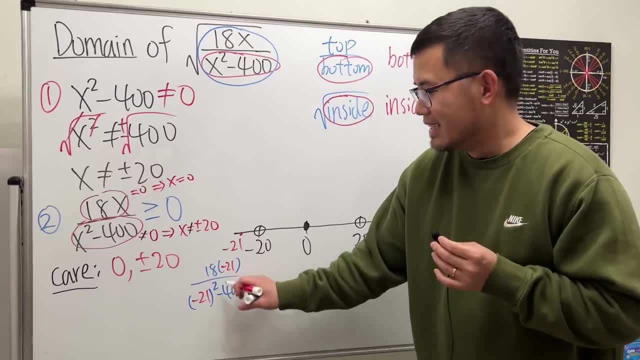 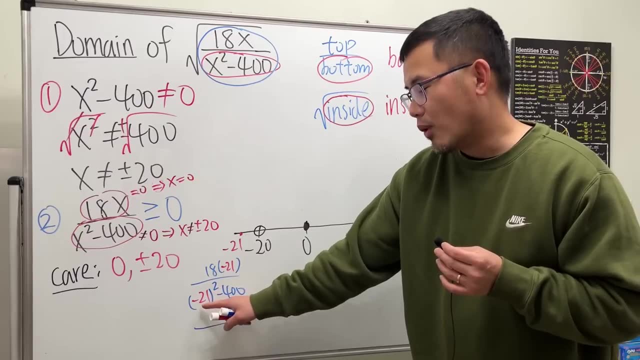 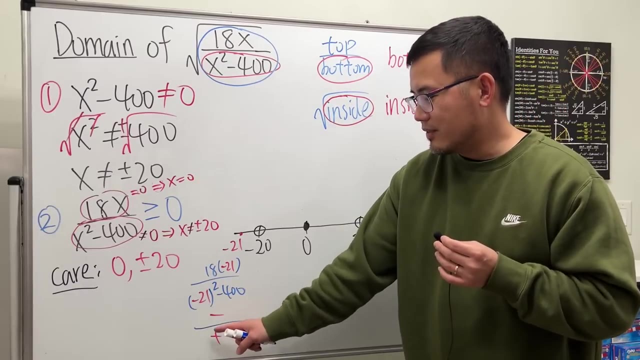 Right here, the top is positive. Oh sorry, Positive times, negative is negative. and then the bottom. well, this right here is going to be 440, something right? 41 minus that. so it's positive. So work that out. You get negative over positive, which all together we get negative. 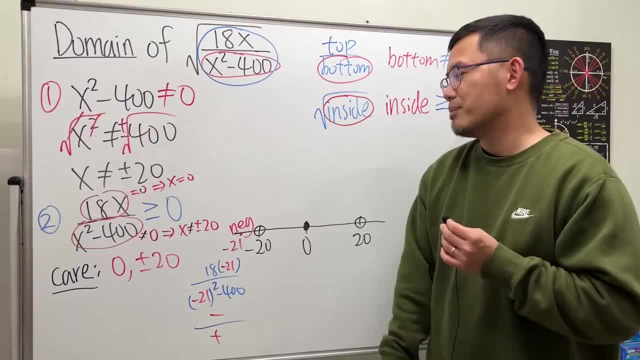 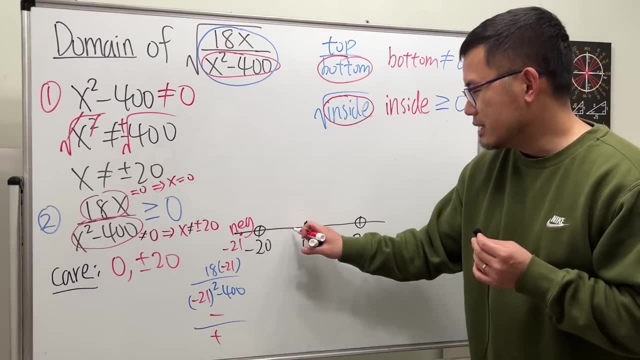 And that's not what we want, because we're looking for the non-negative part. So now go ahead and pick a number from between negative 20 and zero, Let's say 1.. Why not Negative 1, because it's less than zero. 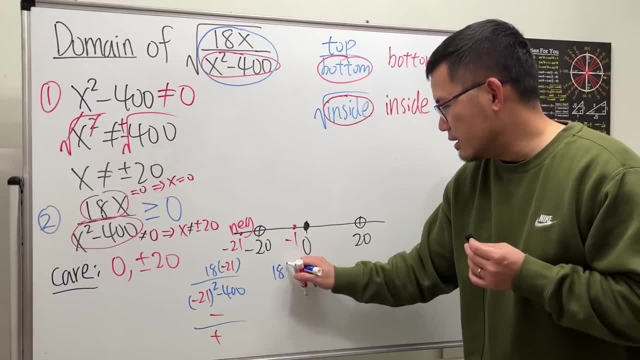 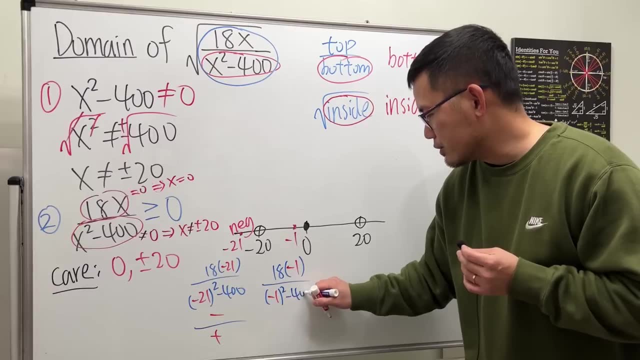 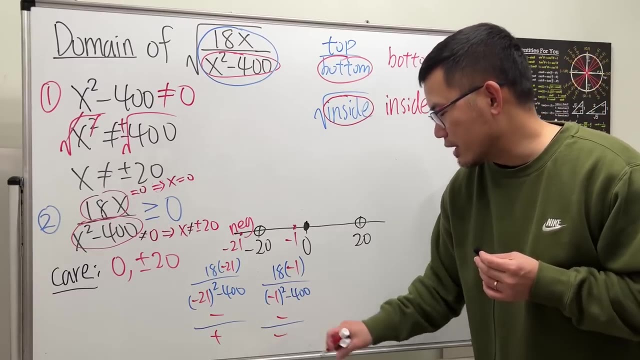 Now put negative 1 into all the x's, We're looking at 18 times negative 1, over negative 1, squared minus 400. Now the top is negative. The bottom right here is 1 minus 400. It's for sure negative. All in all we get. 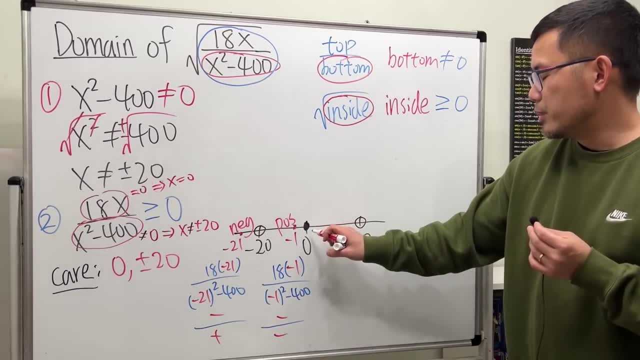 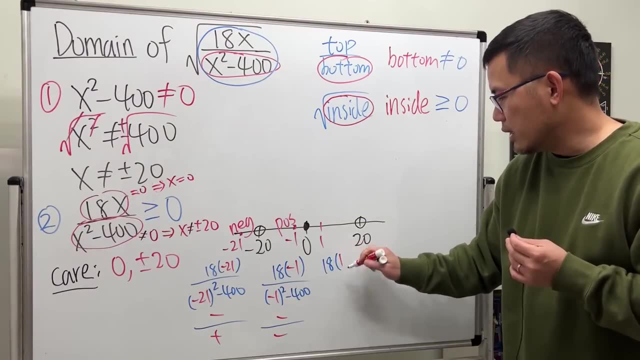 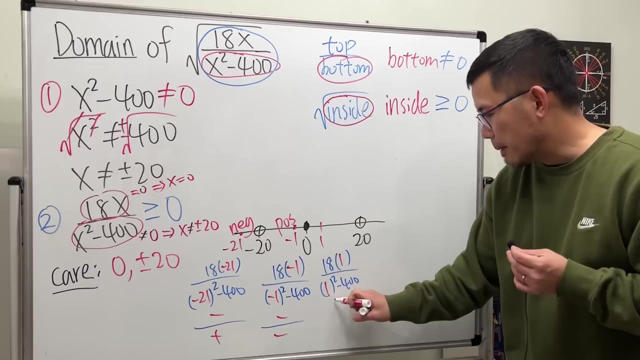 positive. Continue. pick a number between zero and 20, let's say 1, and then put it here. So we're looking at 18 times 1, over 1, squared minus 400. The top is positive, 1 minus that is negative. All in all, this right here is negative and we don't want that section. 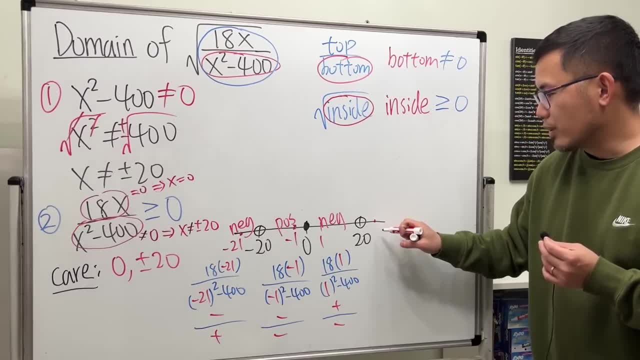 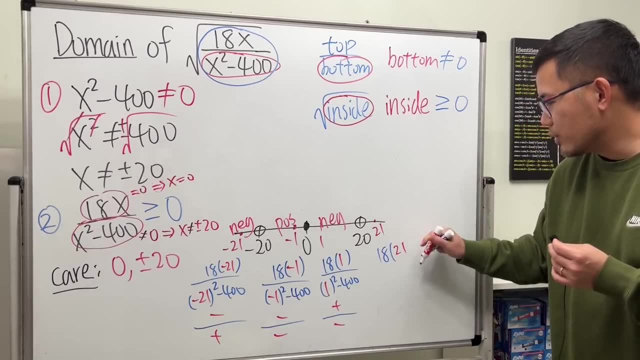 Lastly, pick a number bigger than 20.. Let's say 22. no, don't be too fancy, Just 21. Plug in, so we have 18 times positive, 21 over 21 squared minus 400. The top is positive, The bottom right here. work that out, You will get positive as well. So, all in all, you get positive.